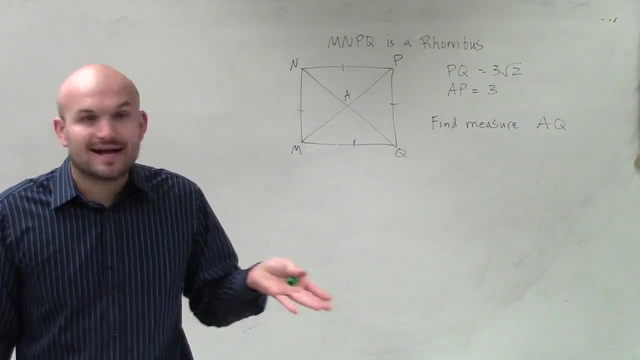 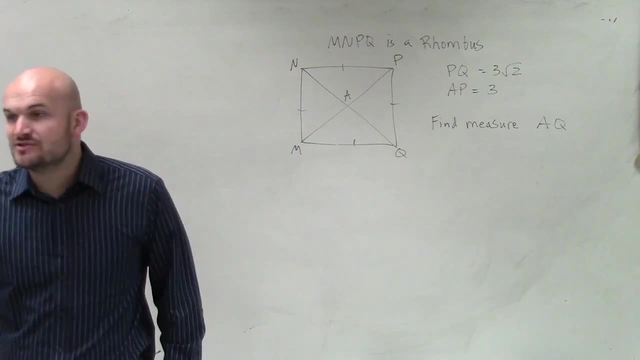 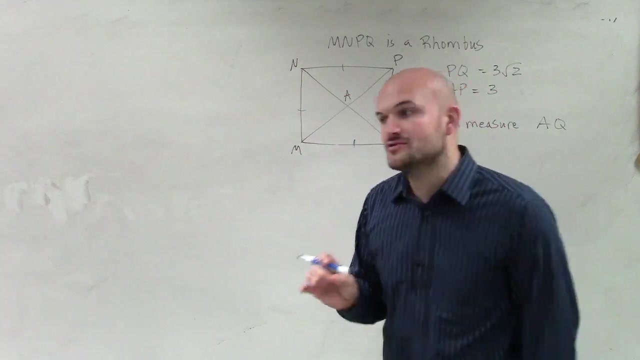 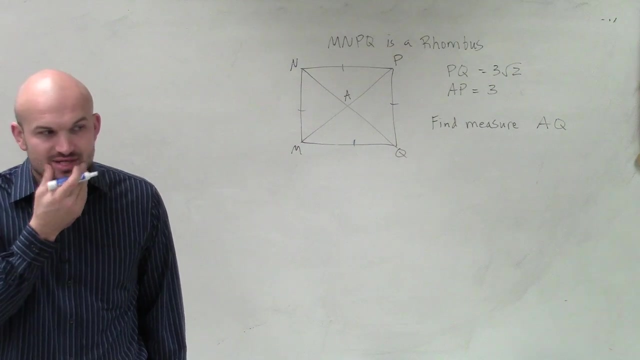 each diagonal in half. However, the diagonals are not equal in measurements like they were for a rectangle and a square, So your diagonals are not always equal, All right, But there was something that was very, very important, AJ. if you just want to flip that over, please, for me There was something that was very, very important about rhombuses, about their diagonals. Does anybody remember on their notes what was very important about the diagonals of a rhombus? Yes, Blake. 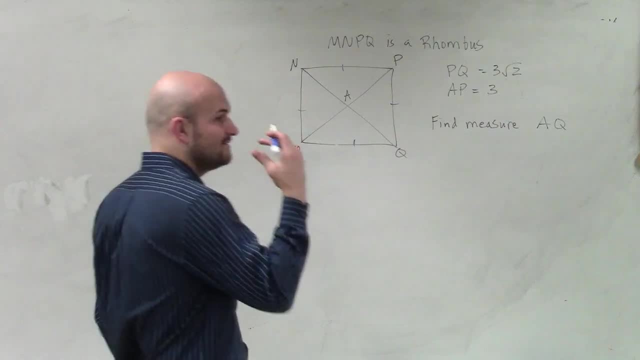 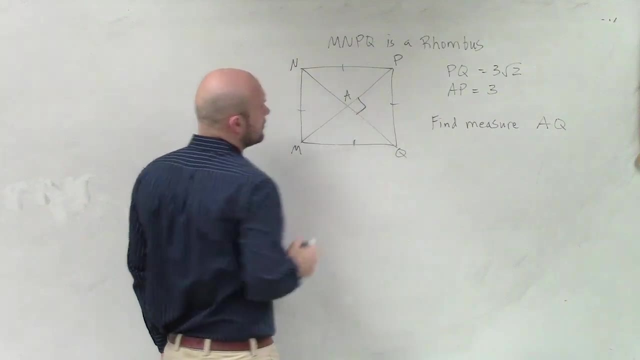 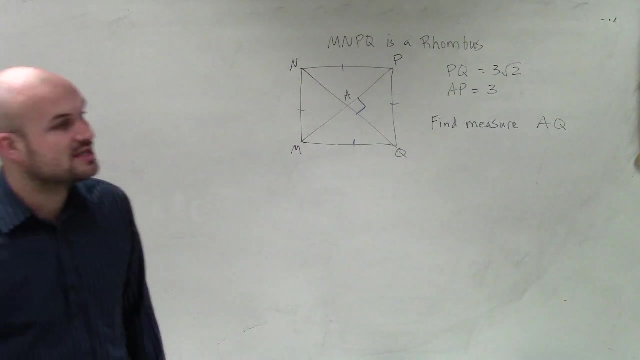 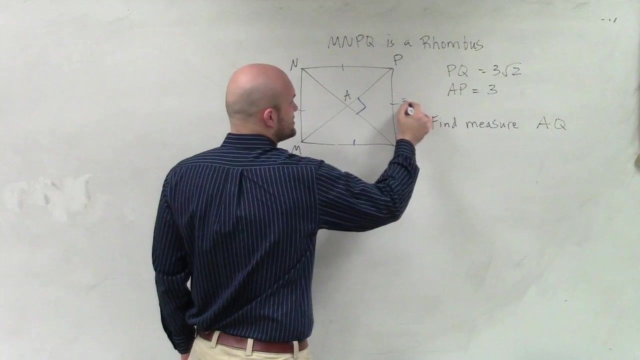 They're perpendicular. So if they're perpendicular, that means they create a A 90-degree angle, A 90-degree angle. So I can write that in for all of them, right? But I'm just going to write it in, right there. So if that's 90 degrees, that means all of those angles are going to be 90 degrees within here. So now let's go and look at what we know. They say PQ is 3 squared of 2, and AP equals 3.. Okay, 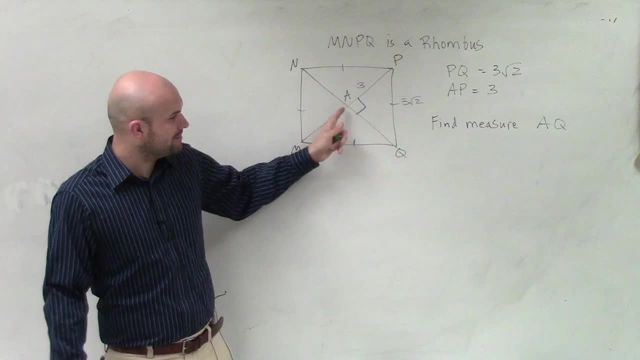 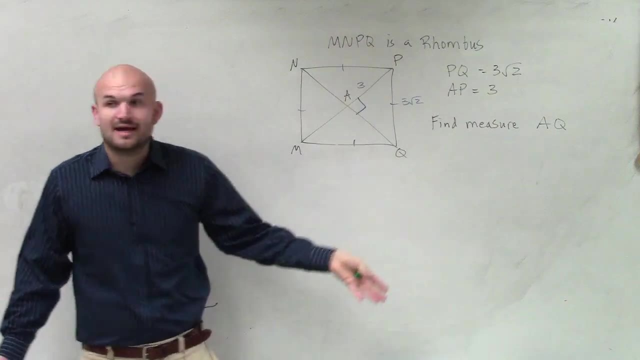 Well, ladies and gentlemen, what is this Now, Phillip? what is this shape right here? A triangle, A triangle? What type of triangle? Remember how we learned how to classify it? It's a right triangle. And when we have a right triangle, what is one of those theorems that starts with a P that we can use? that we just did on our last homework quiz. 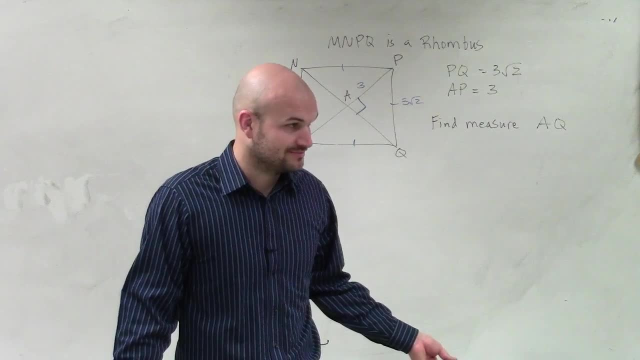 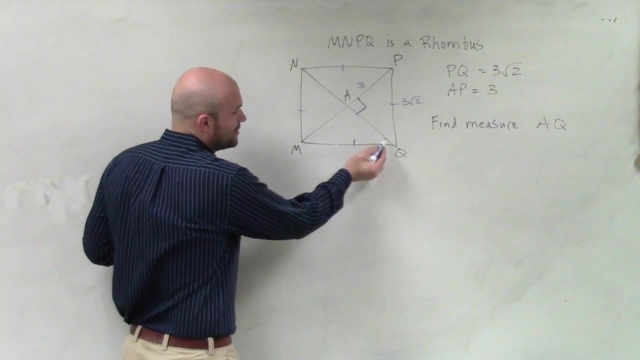 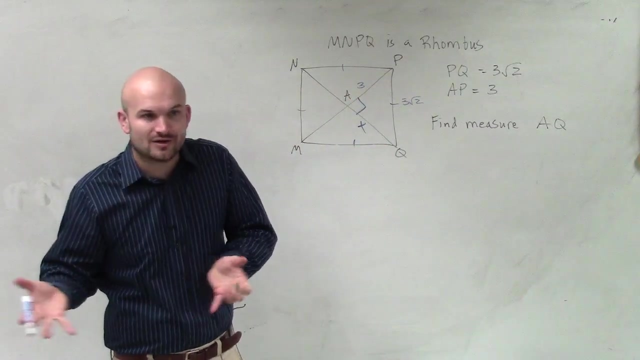 Rhymes. rhymes starts with a P and rhymes with Pythagorean. Pythagorean theorem: Right, We just did this. Right, We just did it. You're trying to find AQ. We don't know AQ. So again, what I tell you guys is: extract the triangle. 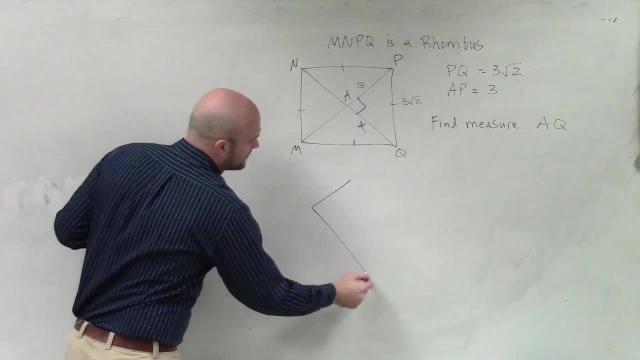 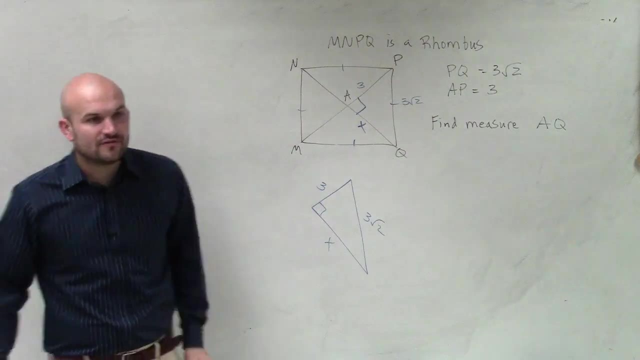 Extract this what you're trying to find. So here's what we have: 3 square root of 2, 3X right triangle. Is that enough information for us to apply the Pythagorean theorem? Yeah, of course it is. 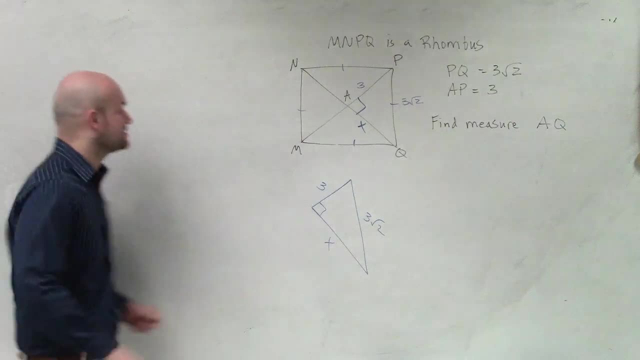 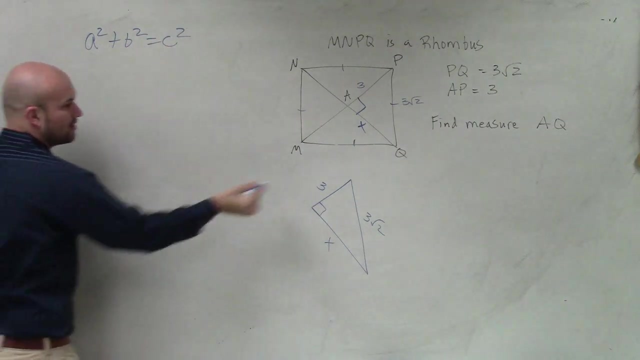 We have a leg and a hypotenuse, So remember, in this case, Pythagorean theorem is: A squared plus B squared Equals C squared. Well, here we'll call that. these are your A's and your B's, right. 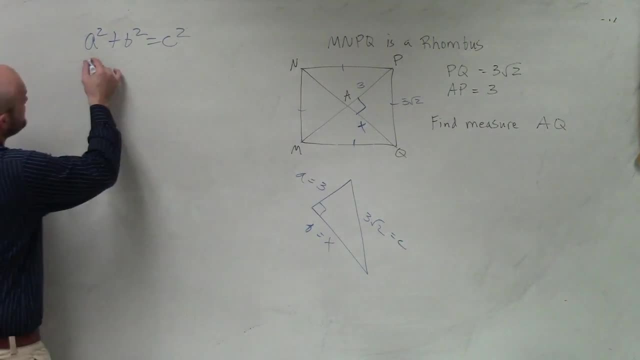 Those are your two legs and that's going to equal your C. So I can say 3 squared plus X squared equals 3 square root of 2 squared. Now I know we haven't dealt a lot with the radicals, all right. 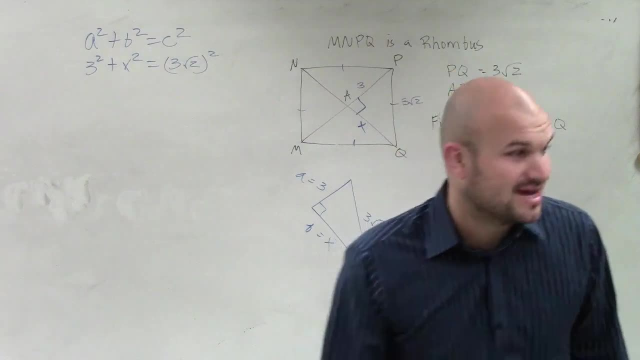 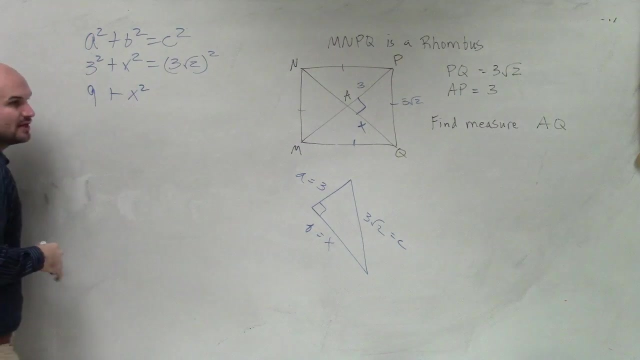 So I can fully understand if you guys had some problems with this, But you guys have been introduced to radicals before. 3 squared is going to equal 9 plus X squared 3 times Times square root of 2 times 3 square root of 2.. 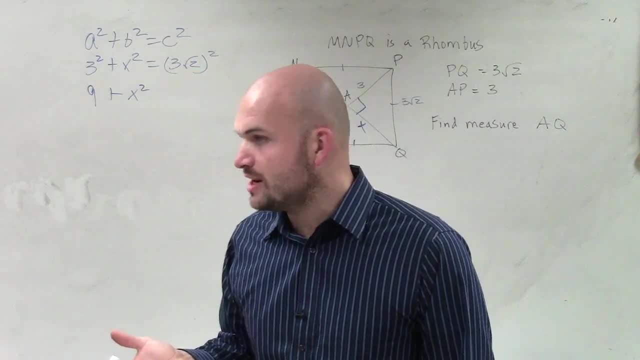 Well, square root of 2 times square root of 2 is square root of 2 squared, which is just going to be 2.. 3 times 3 is going to be 9.. 9 times 2 will be 18.. 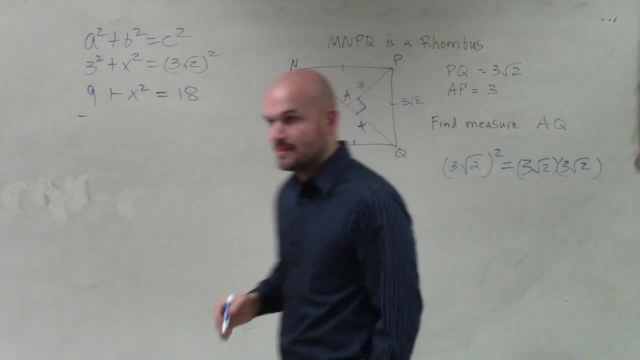 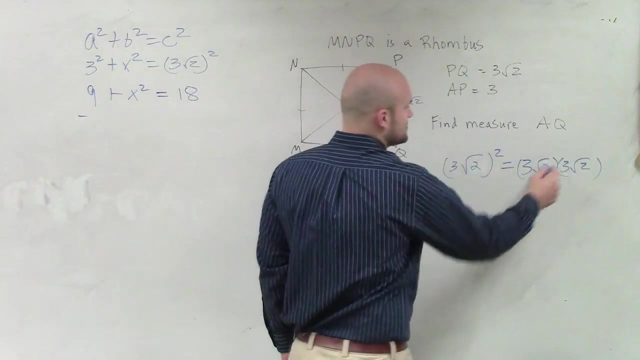 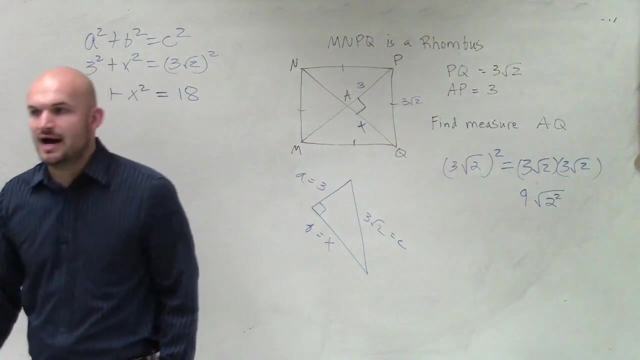 Would you agree, Do you guys agree, that something squared means that multiplied by itself, right 3 times 3 is 9.. Square root of 2 times square root of 2 equals the square root of 2 squared right. The inverse operation of adding berta is: 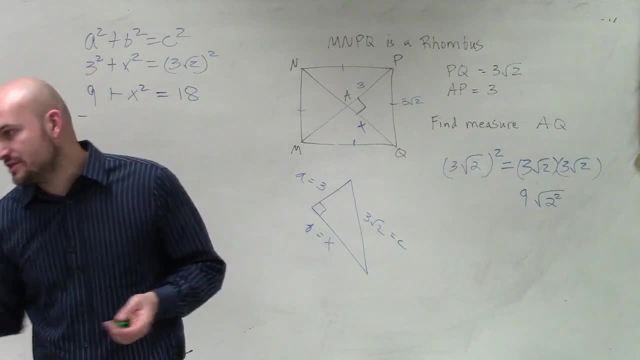 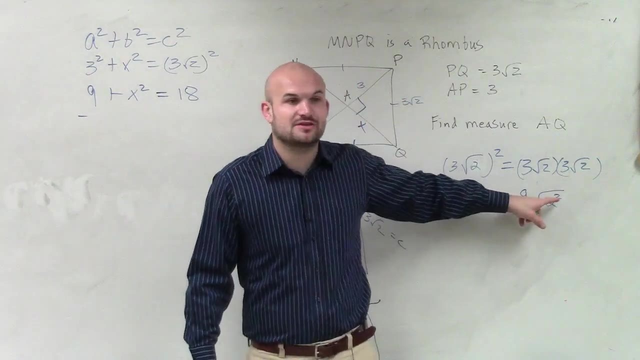 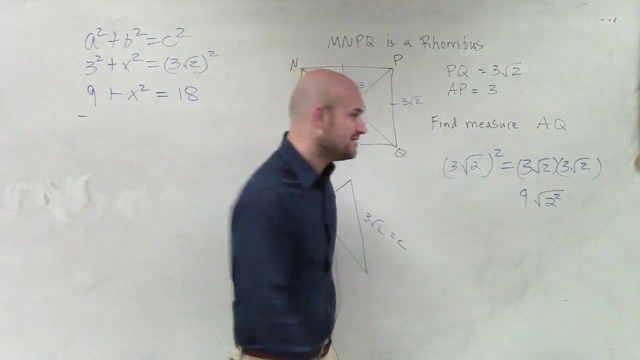 Subtracting The opposite operation of division: Samantha is multiplication right. The opposite operation of taking the square root: Sierra is squaring right. These are opposites, So therefore those undo each other and you're just left with 18.. 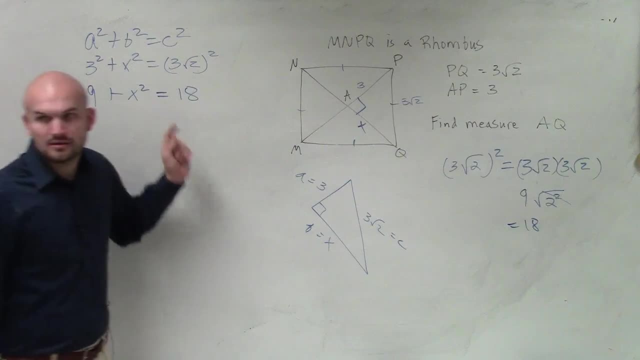 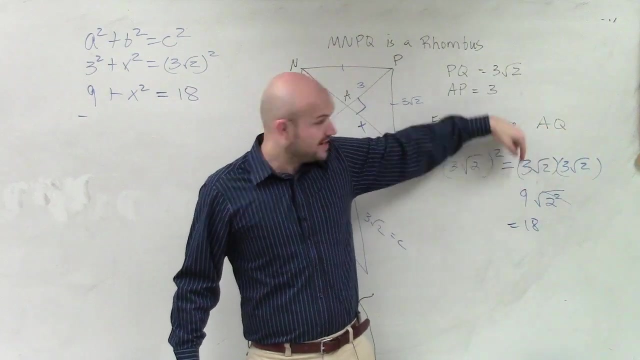 So that's what I said out loud in my head and that's where I got that. Does that make sense, AJ? No, Do you understand? this equals that? Yeah. Do you understand? 3 times 3 is 9? Yeah. 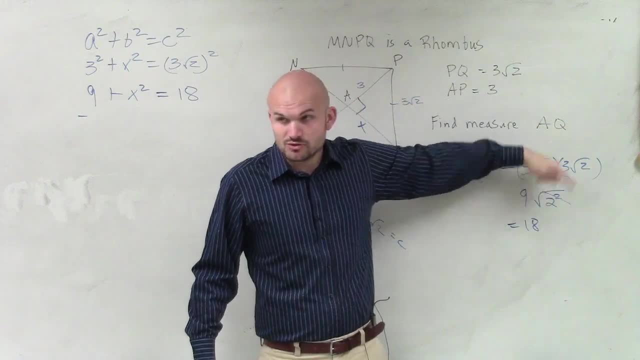 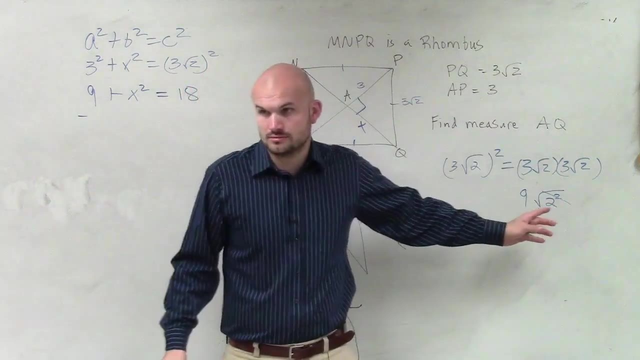 Do you understand? square root of 2 times square root of 2 is just going to be 2 squared. Square root of 2 squared, Right? No, you don't. Square root of 2, 2 squared and then the square root and squaring, those are opposite of each other. 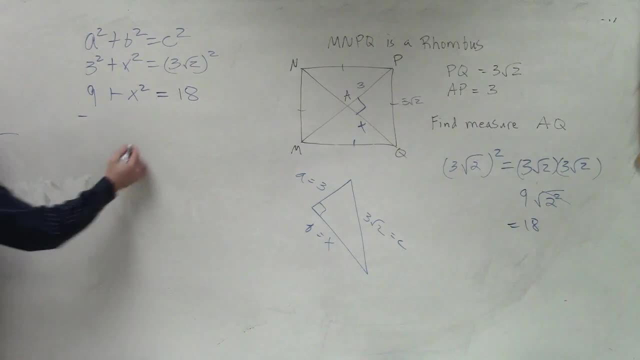 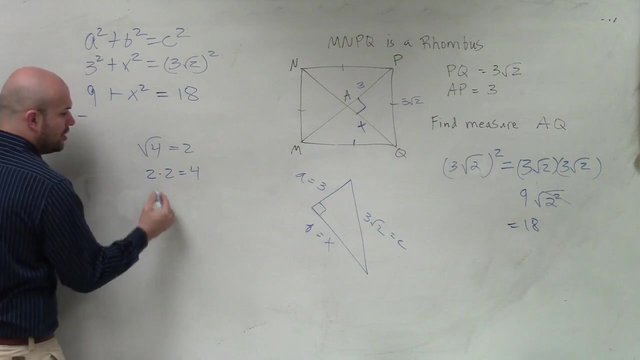 Those are opposite of each other, like right. What's the square root of 4? 2.. Why is it equal to 2? Because 2 times 2 equals 4, or 2 squared equals 4, right. 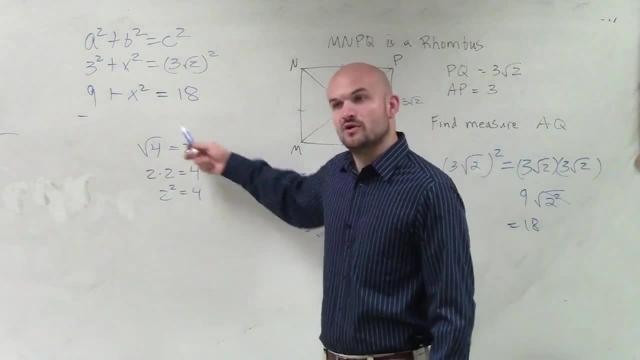 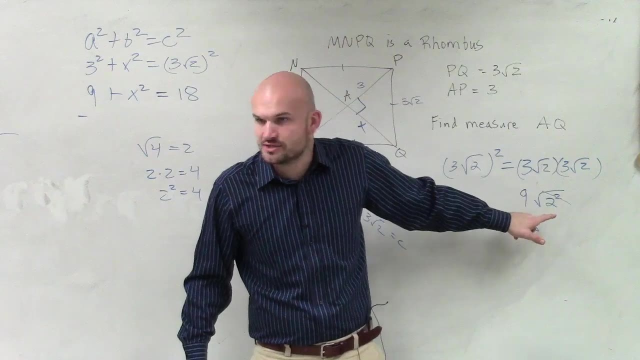 Those are opposite of each other. 2 squared equals 4, square root of 4 equals 2.. Those are opposite. Those are opposite operations. So if I have the square root of something squared, that's just going to equal my radicand, which will be 2..